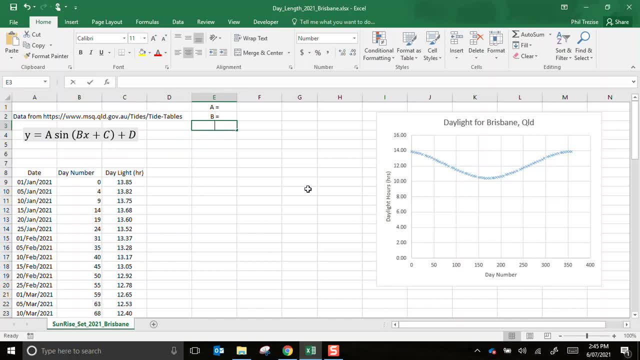 numbers. I don't know what the numbers are yet, but that's the goal, if you like to find the right set of numbers. So I'm just going to set up some data cells here- a, b, c and d- and just to begin with, 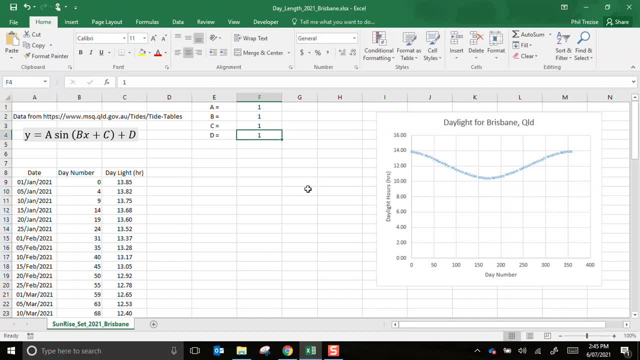 so that everything works. I'll put the numbers: 1. To make them stand out, make them a little bit special. I might put a little bit of shading by behind those and those numbers. there I'm going to change. In a minute I'll make a. 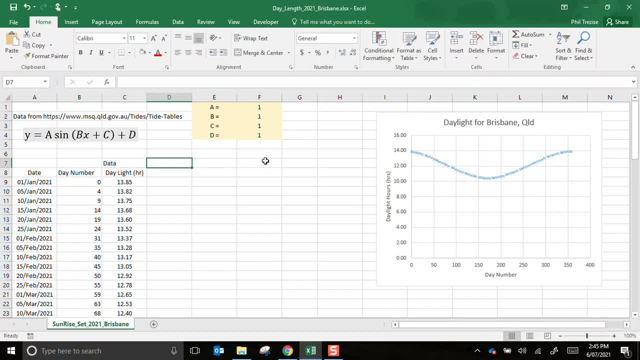 note that this column is my data and this column is my model, my mathematical formula, if you like. So what do I need to do with this? Well, I need an Excel formula that looks like a by the sine of bx plus c plus d, where 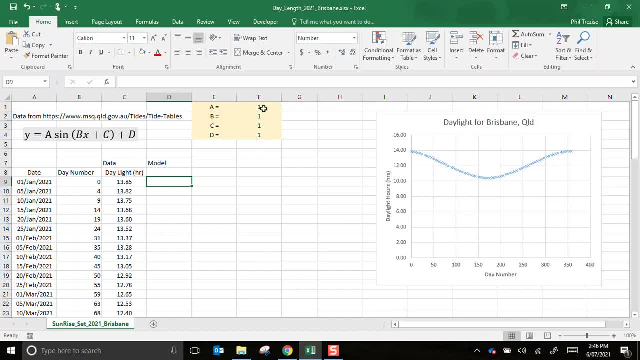 I refer to the value of a, b, c and d from up here. So let's see if I can do that. I'll start with an equal sign Where it says capital A. I'll click on that cell and again I'll press the F4 key to make that an absolute reference, because I 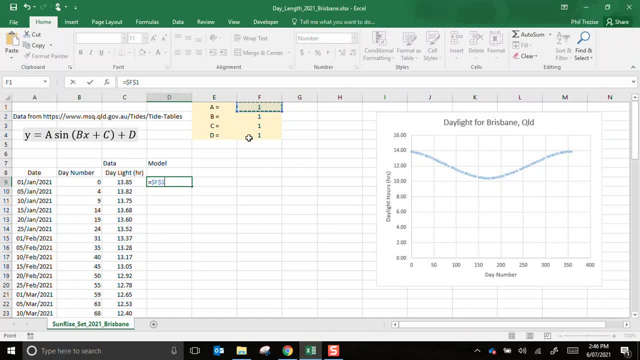 always want the a, the b, the c and the d to be from these four cells. even when I copy down the page, Asterisk is multiplication. Then I type sine. that's fine, Open my brackets Now. I would normally start to go b, x plus c at this stage, but I do have to. 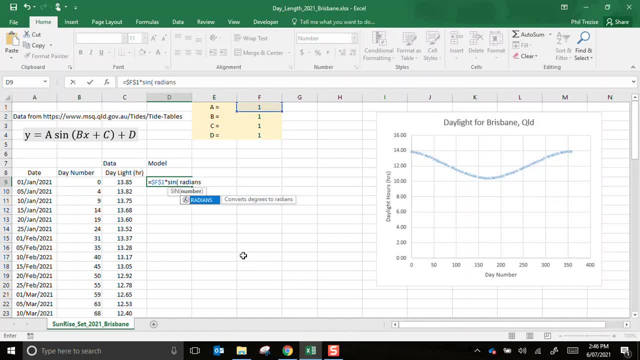 warn you that Excel works in a measurement called radians for angles. Now you'll learn about radians when you're in grade 11, but at this stage we will just use the built-in function radians to convert angles from degrees into the measure of radians. 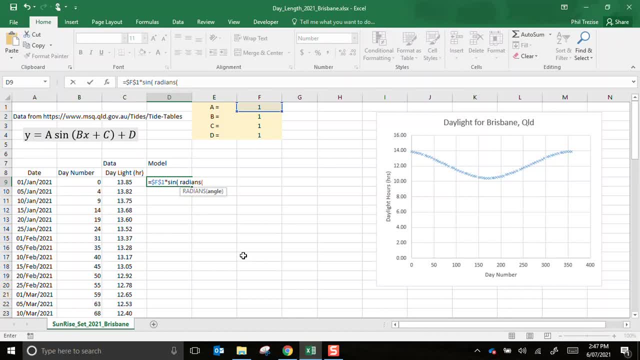 So we'll just go with the measurement that Excel needs. It's a bit like converting from kilometres to miles. as long as it's taken care of, everything works. We don't need to know the details at this point in our lives how that works, but it's needed for Excel. 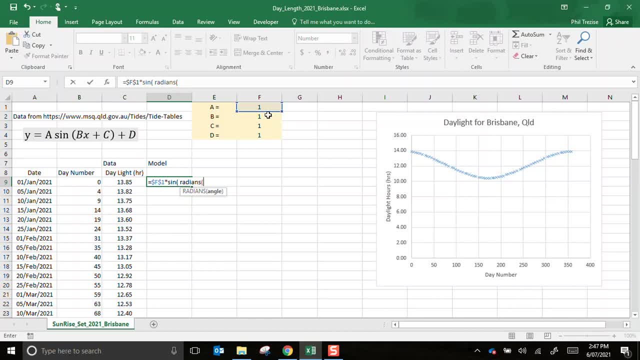 So now I'll put: I'm up to the bx plus c, So there's b, F4 again multiplied by now see that the x here is a lower case letter. so is the y. These are the variables. So what is the x value? Well, the x values on my chart are the day numbers, and in 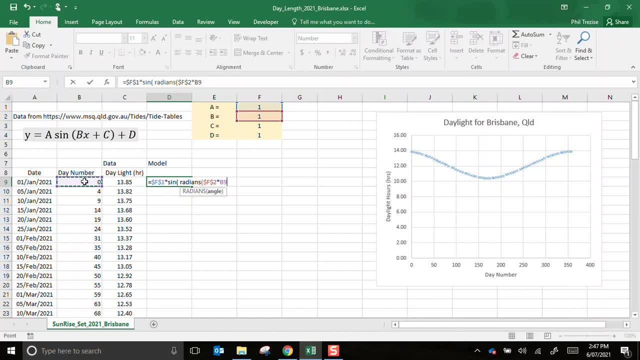 this particular case, that would be the number zero. In other words, sell B9.. I am not going to put dollar signs on B9.. When I copy this formula downwards, I want the next row to be looking at B10 for the x value, and then B11 and so on. So that's the x. Now I have to go plus c Again. that's a. 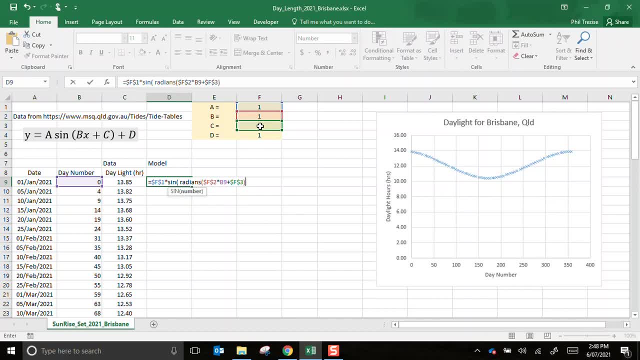 fixed constant. I close the brackets. Notice how they flashed red for a moment. That's the radiance function. I close the brackets again. That's the sine function. and now I put plus d, which is that one there, and I press f4.. Now, apart from the radiance part, 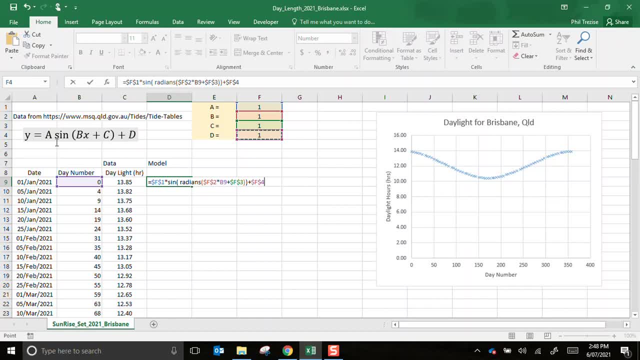 it looks almost identical to this, where the a, the b, the c and the d are replaced by the references to these cells. When I press enter, I get an answer which is nowhere near what I wanted. I want the numbers in this to match the numbers here. Now. don't worry too much at this stage, I'll double. 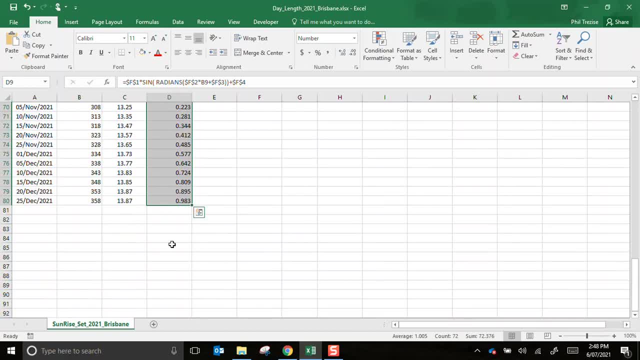 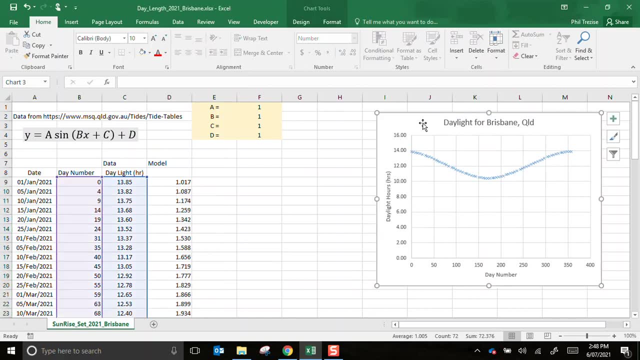 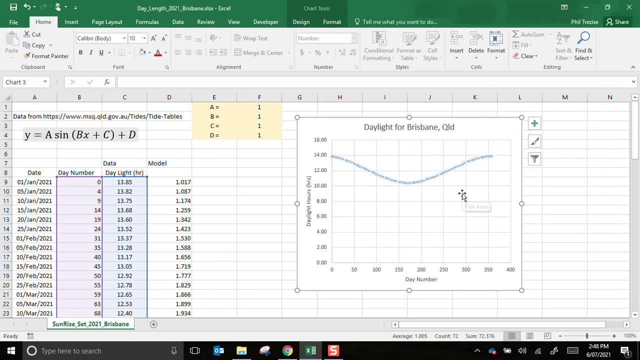 click there to copy those down, and there is a set of numbers which is not going to match. I get that, But we'll adjust. Now I'll bring this back over. I'm going to add this set of numbers to my scatter chart, So notice. I've clicked on the chart, Go up to the design tab, Then select data. Now I'm going. 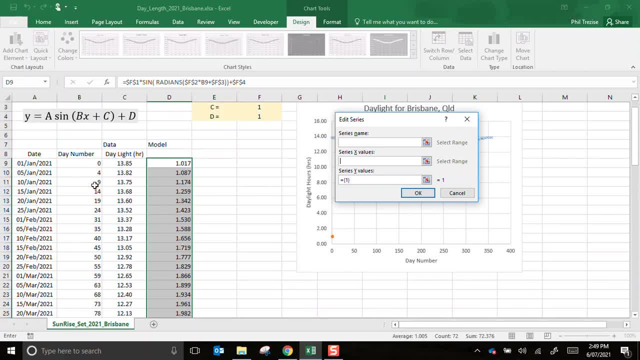 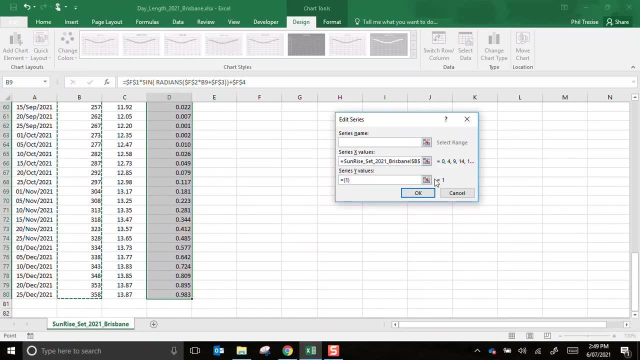 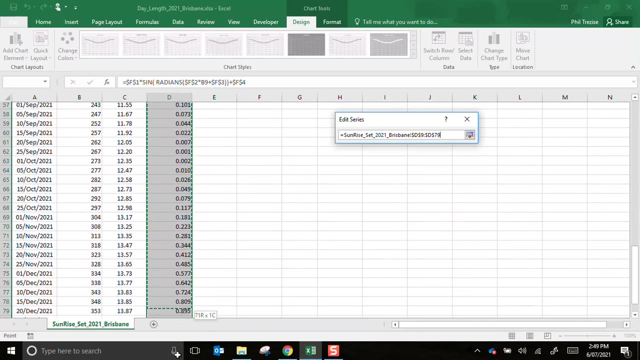 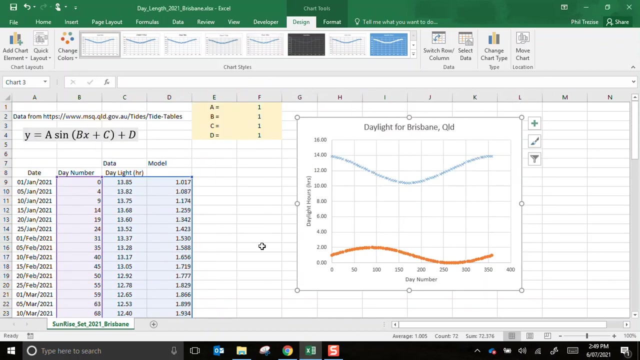 to add a data series. The x values are the day numbers from 0 to 358.. The y values are these new numbers here. OK and OK. Now, it's nowhere near what I need it to be, But at least it's there. And once it's there I can start to adjust my 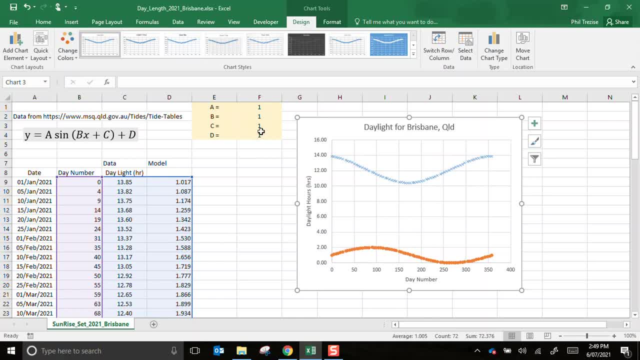 values of a, b, c and d. These are the parameters. If I adjust the parameters, this will change Now. before I get too detailed into that, I need to add values of a, c and d. These are the parameters. If I adjust the parameters, this will change Now. before I get too detailed into that, I'm going to need to find the values of a, b, c and d. 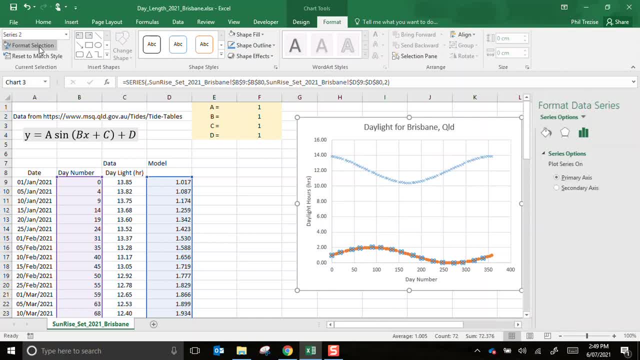 I'm going to format that data series, series number 2, and again the little thing that looks like a bucket of paint. This time I will have no markers. I don't want dots or X's. I'll say none for the markers. 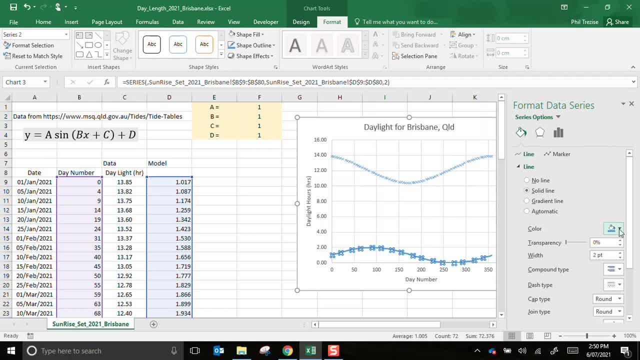 And before I lose it, I'll go across to the line. I'll have a solid line, and the orange is a nice contrasting colour and let's make it about 1.5 points, so it's a nice thin line. Now the fun begins. 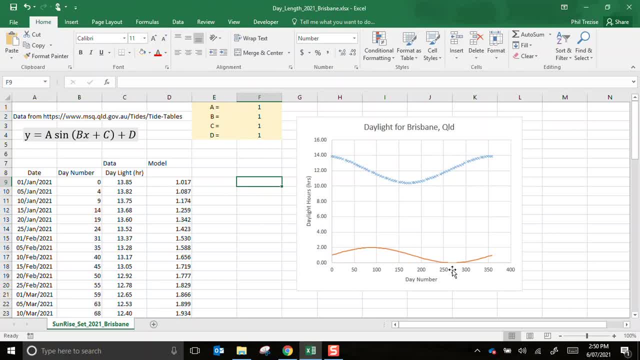 I get to change the numbers A, B, C and D until the orange line matches this one. I think it's easier to start with D. Remember, D represents the equilibrium value. Now, the equilibrium value for mine here looks to be about 12, so I'll put 12.. 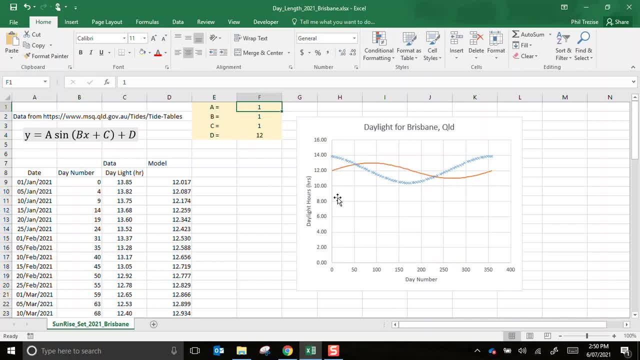 And there we go. that's not too bad. Now I'll go to A. A represents the amplitude, so from the equilibrium to the maximum looks to be upwards by about 2, and from equilibrium to here looks to be downwards by about 2.. 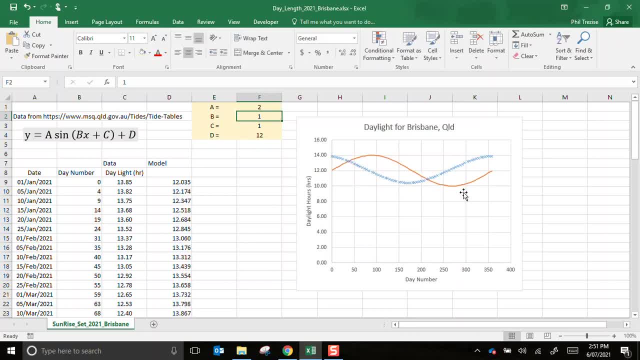 So I put 2, then, OK, that's not too bad. Now I've got B, represents is a measurement that controls the wavelength. The wavelength looks about right because I've got- almost I think I've got- about one cycle here for my blue data points and that's pretty much one cycle as well. 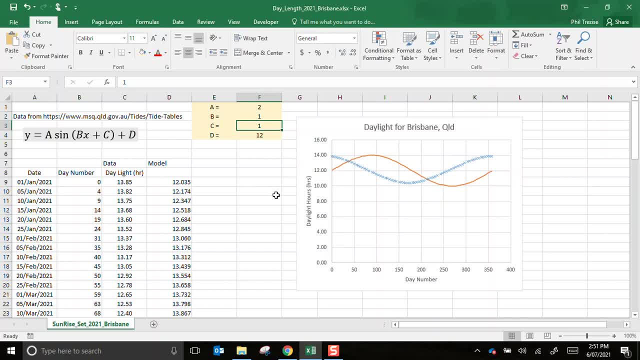 So I think that's OK. C is the phase shift. It will slide my orange line to the left or to the right. Let me just try making that one. let's make that about 90.. Pretty close, not too bad. Maybe I need to go a little bit more. say 91..